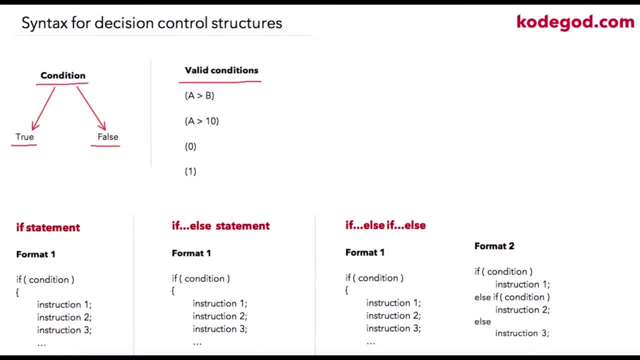 conditions: a greater than b, a greater than 10,, 0 and 1.. Now how these are valid conditions. All the conditions are evaluated to a certain value. If value is 0, the result is false And if the condition is evaluated to any non-zero number, it will be treated as a true. In this case, 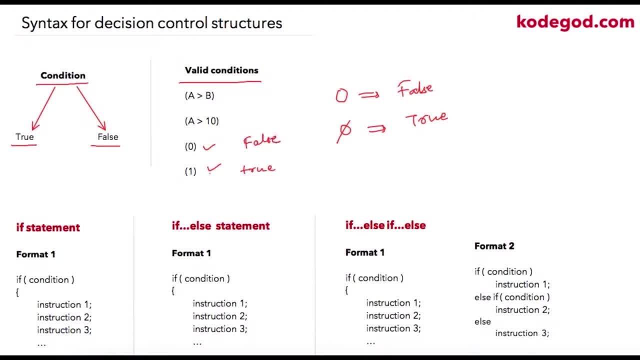 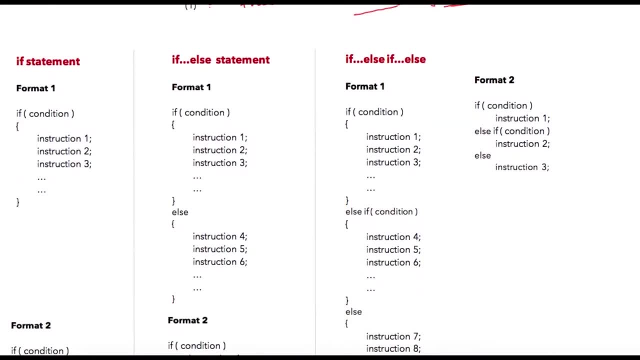 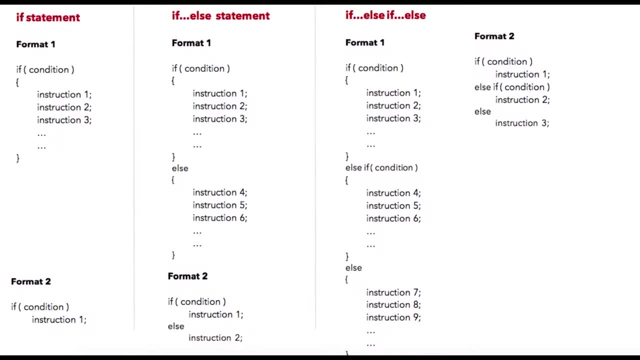 1 is true and 0 is false. Similarly, minus 100, little constant a- all these values are true. Now let us check the syntax. So this is general. if statement Format 1, as an example, is: if inside of parenthesis I am writing condition, If the condition is true. 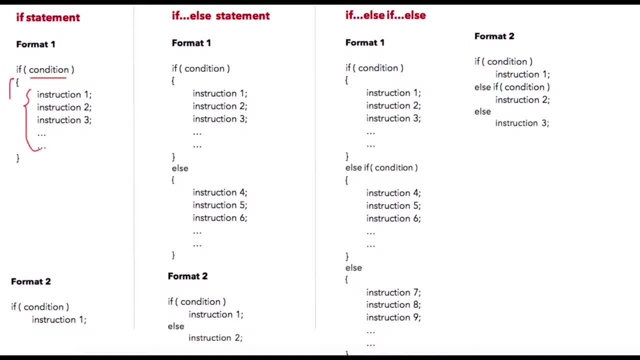 all these instructions will be executed. This whole part is my if block. If my condition is false, this whole block will be skipped. Format 2 will not get executed at all. Now let us talk about format 2.. If my if block has a single 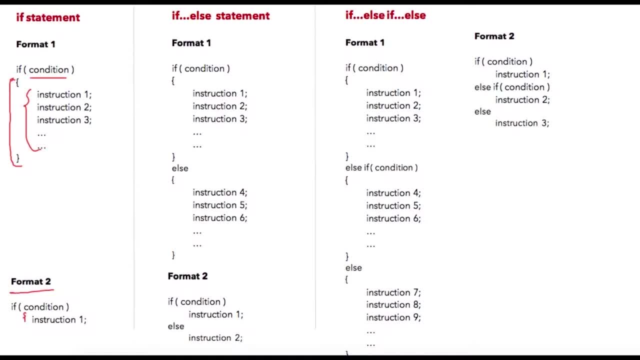 instruction. I can exclude writing curly braces, So we can just simply write my condition and the instruction. So this instruction will only get executed if the condition is true. Now we will check if else statement. So similarly like if, whole format for if is same. But what we will do. 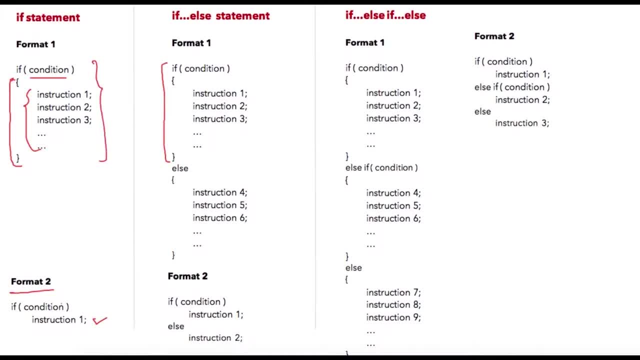 here is only if. If my condition is true, some statement will get executed. However, in case of condition is false, we were not writing anything. So if you have those kind of cases, we can write else, block Okay. so if my condition is true, this whole thing will executed, Else, these statements will get. 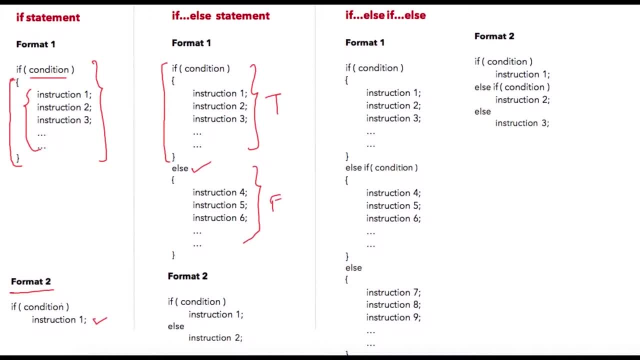 executed. Similarly, if we just have single, single statement for if else, so there's no need of writing curly braces over here. Just simply write: if condition your instruction one, else instruction two. we can also write if else as a nested conditions, Like this: I'm writing: if block, then this is my else block, So after this else.